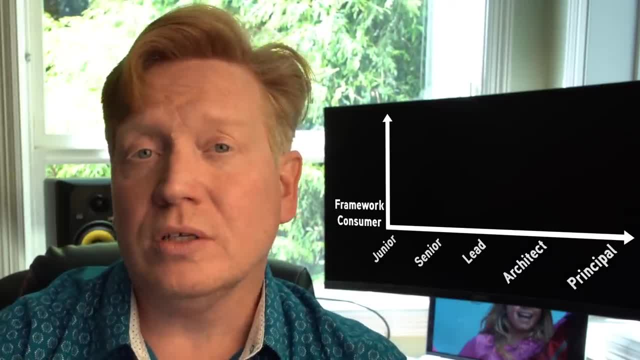 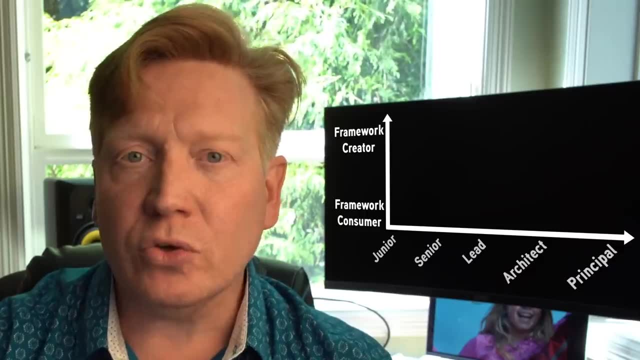 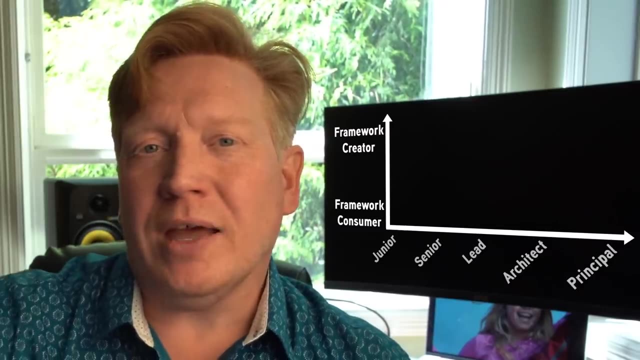 as going from a framework consumer to a framework creator. So you start off using something like Spring or React or Vue, depending on the paradigm within which you're working, And you are moving up that technology proficiency chain, from where you're actually just consuming that framework to 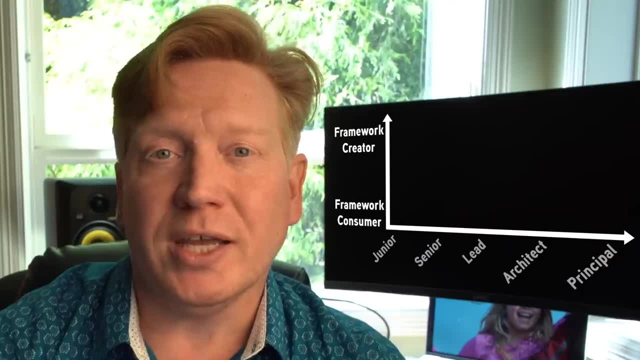 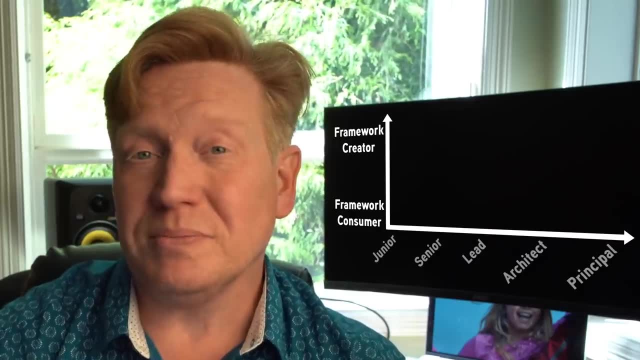 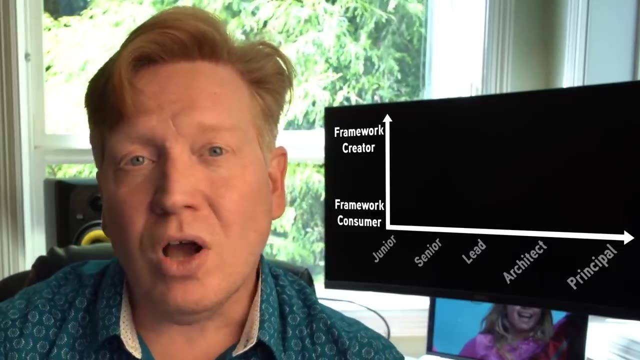 where you're ending up creating a framework that is used by tens, hundreds, thousands, tens of thousands of other engineers, And they become your consumers. So to get there, you have to build up your technology, your skill set right And you start off with basic proficiency in your language of choice, and be it, you know. 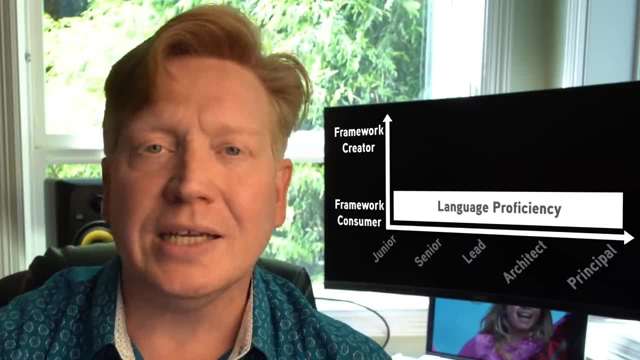 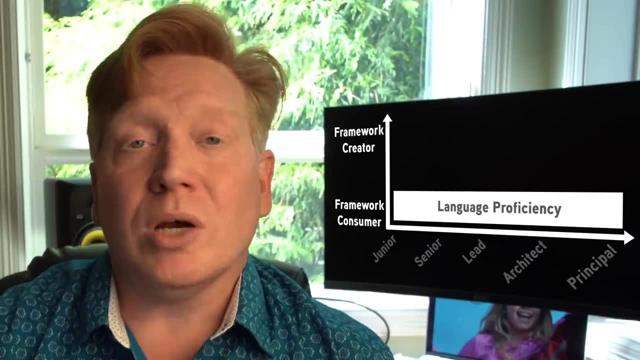 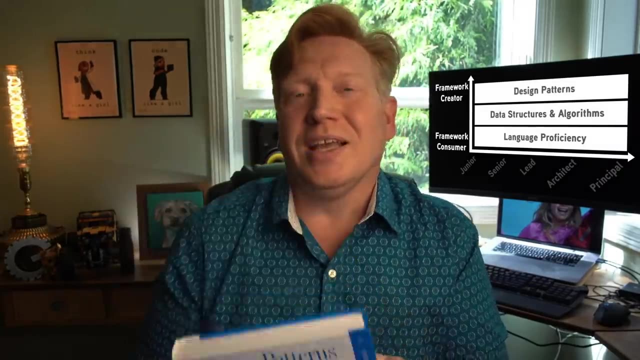 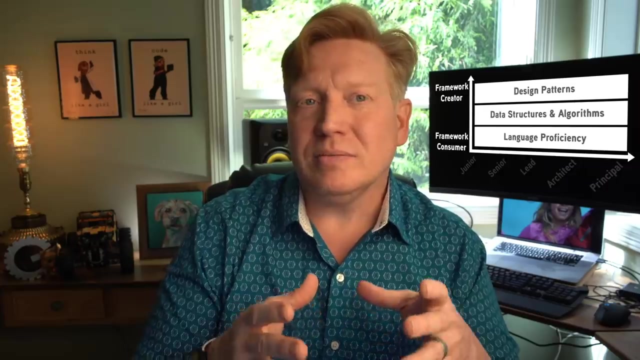 learning about all the ways of doing conditionals and looping and creating functions and methods and classes and instantiating objects and all that Then you work up to data structures and algorithms And finally into design patterns, And design patterns are ways of expressing solid architectures that are reusable and 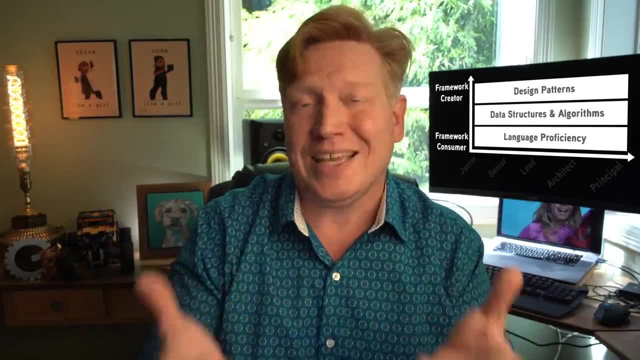 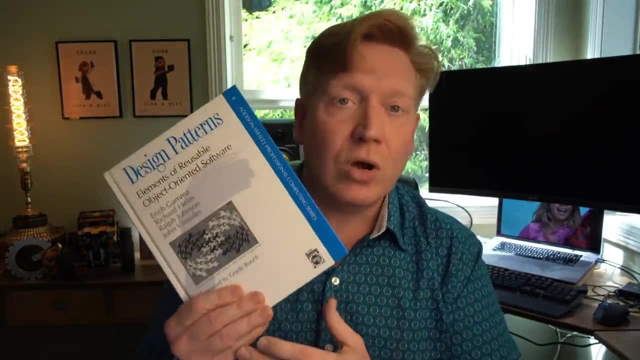 extensible and that are industry standards. So in this video we're going to look at five different design patterns from this, the original OG book, the Gang of Four Design Patterns book. It is in C++ but the concepts are you know, it's a little bit different And it's a little bit different from the 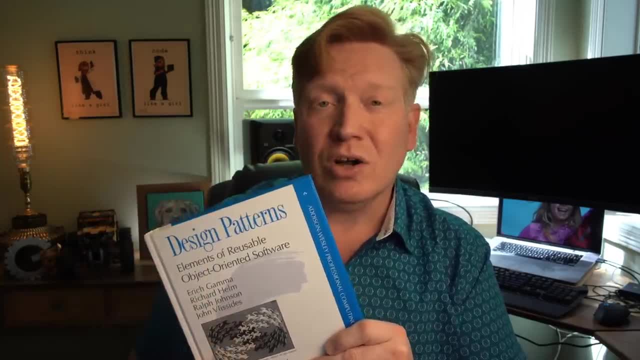 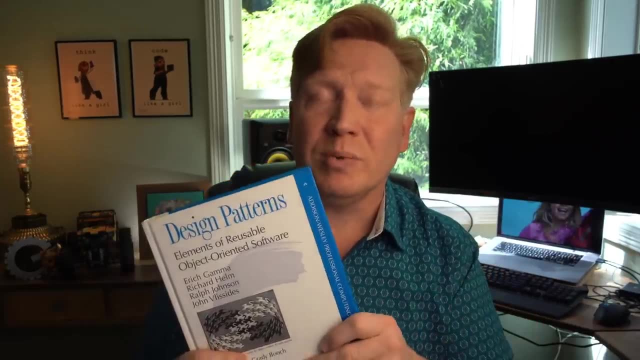 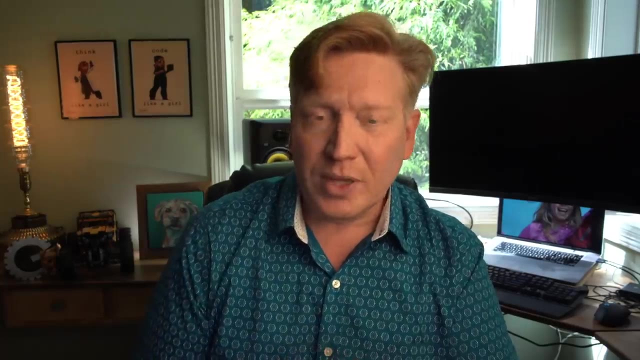 original right, But the concept is that design patterns are usable and understandable in any language and also in any environment. So, on the browser, in Android or iOS, on the server, wherever you're going to be, design patterns are going to help you go from a framework consumer to a framework creator. All right, let's 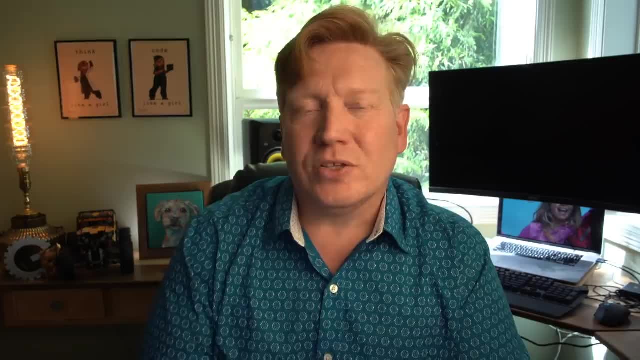 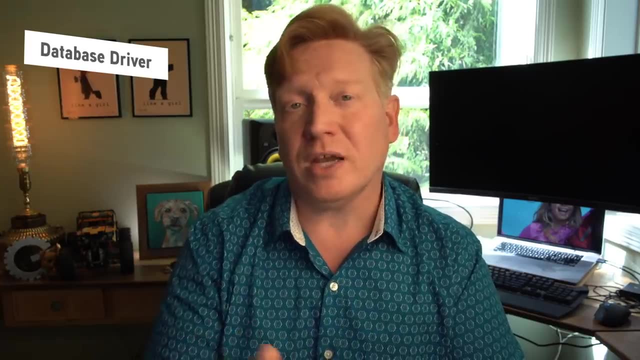 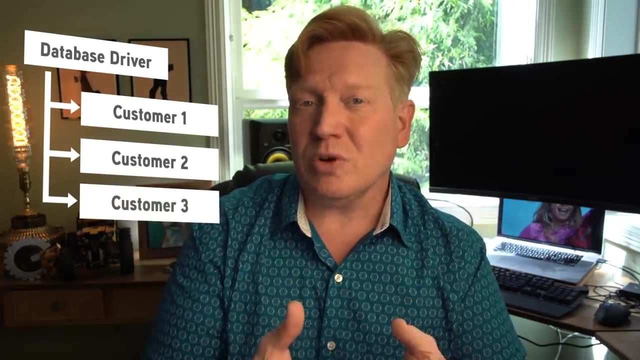 start off with our first one and let's see how fast can identify it. So you have a database driver that you're connecting to. You want to get a list of all of your customers, so you make that query and you get back a list of all the objects which are customer objects. so in this case you've got the customer. 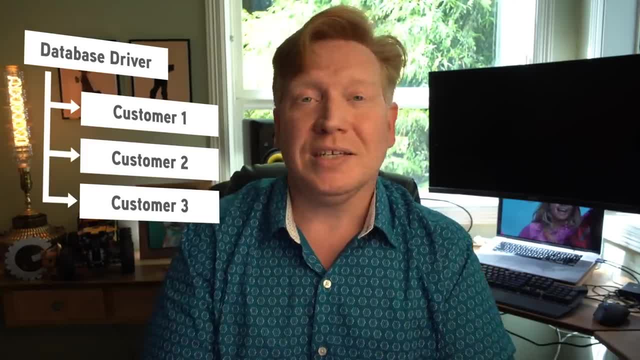 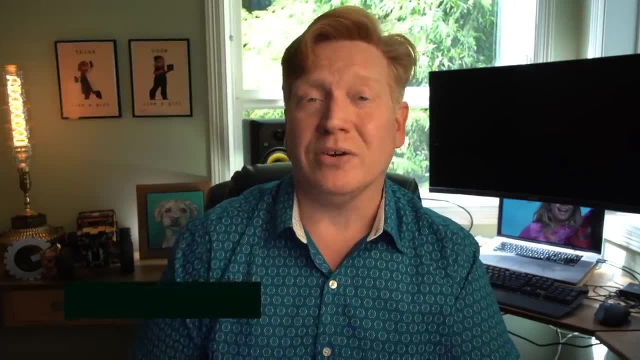 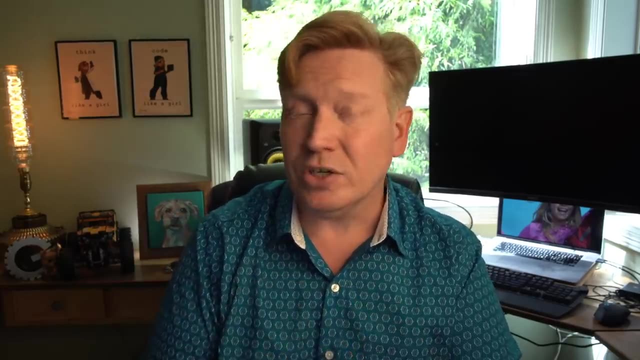 object or the customer class, of which you can have many, and then the database driver, of which there can only be one. and you might have guessed it, that's the singleton pattern as specified in here, and it means that for that given class there can only be one instance, and that's really good for. 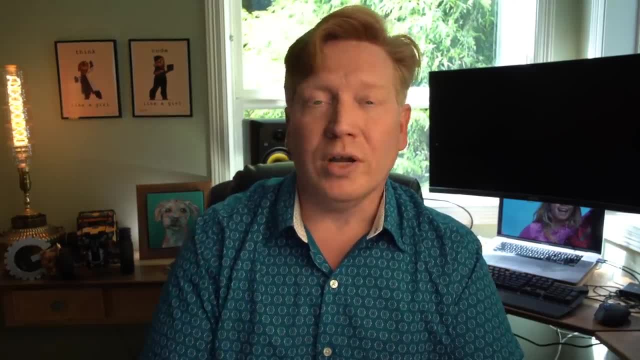 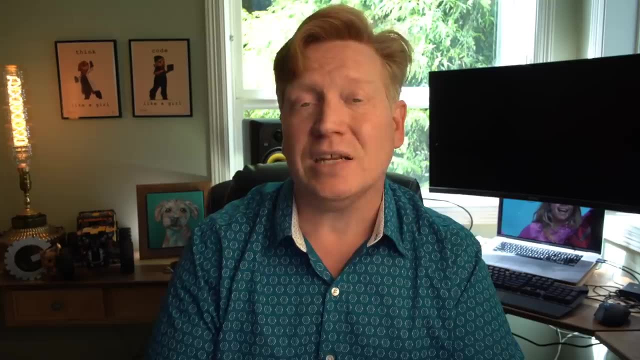 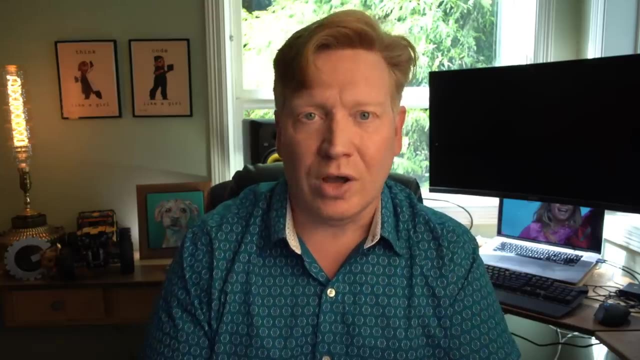 doing things like a database driver or the list of all the configuration settings for your application or, if you're over on the client, maybe the data store, the current state of the app. that's stored in a singleton. the pro is that you can go and get to that data anytime that you want. 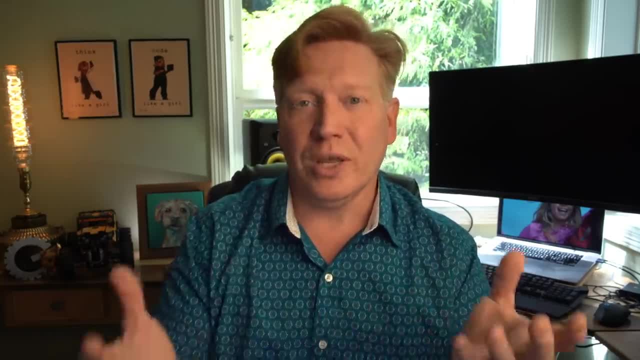 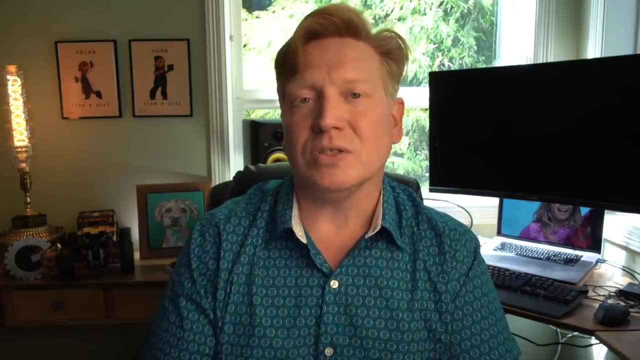 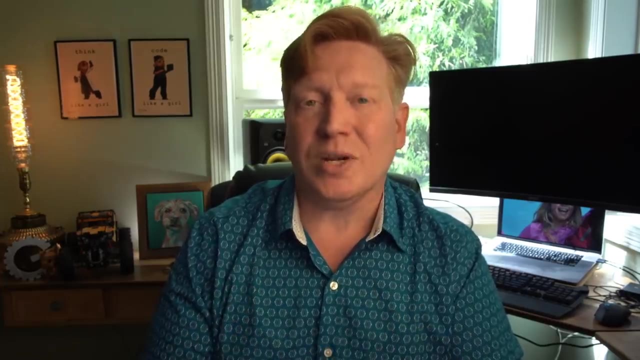 all you have to do is just, you know, get the singleton and away you go. the con in your evolution to framework creator is you might jump on the singleton bandwagon too early and once you've gone there, once you've said that there can be only one and you've added that constraint, it's. 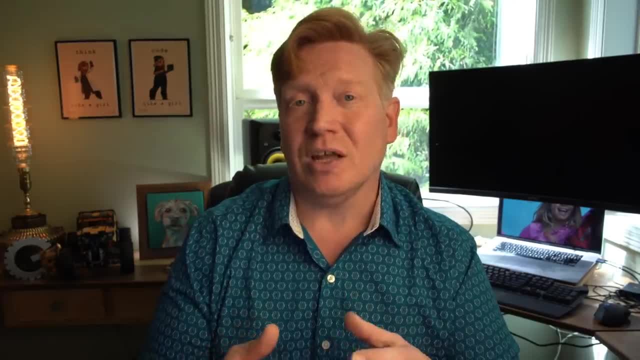 really hard to do anything and you're not going to be able to jump on that and it's really hard to. And once you've said that there can be only one and you've added that constraint, it's really really hard to, really hard to back that out. It means that instead of everybody being able to just go and 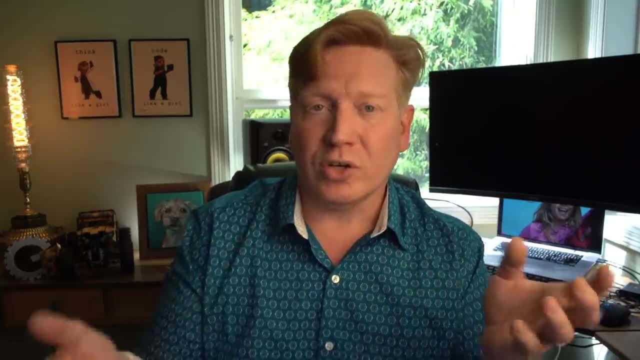 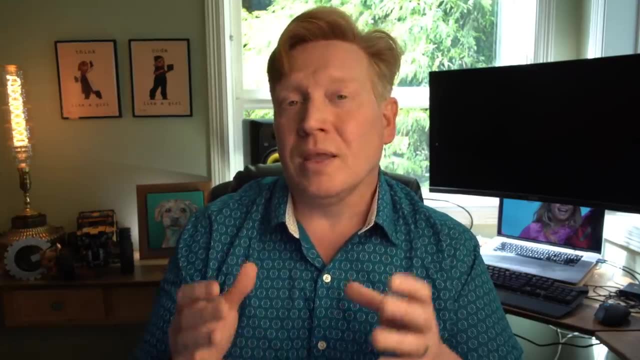 access it directly. now you've got to pipe down whatever the current database driver in this case is an example. You got to pipe that down to whomever the consumers are. So, as with all of these design patterns, you got to make sure that you're using it the right way and at the right. 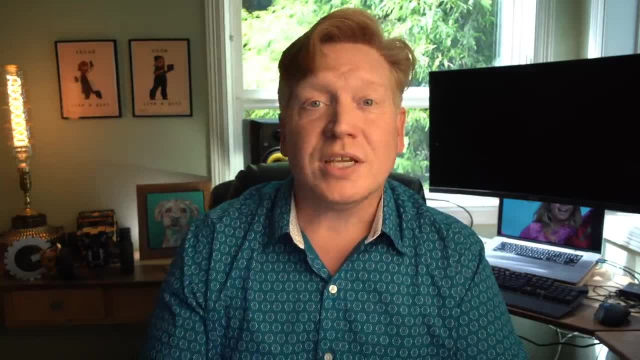 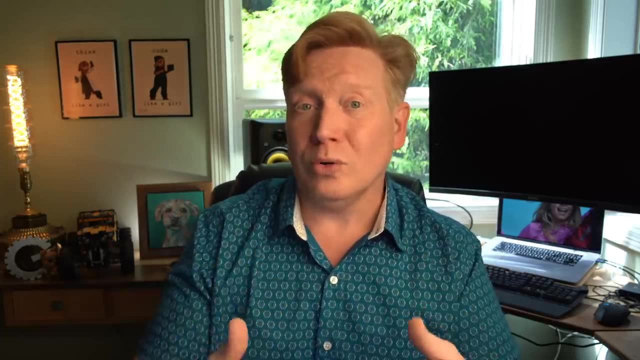 time, Otherwise you're going to get stung. The second design pattern we're going to look at is the facade pattern, And a lot of these design patterns are actually modeled on real world building style architecture, And this is no different. So a facade in the real world is the. 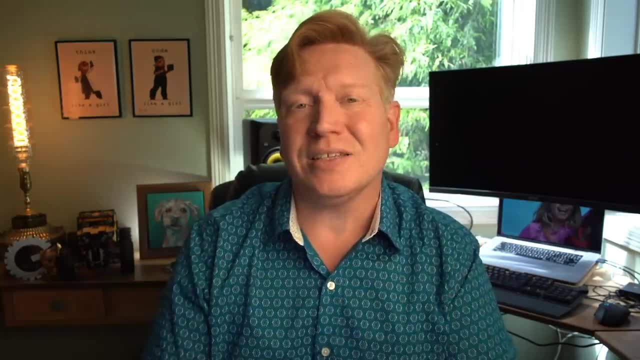 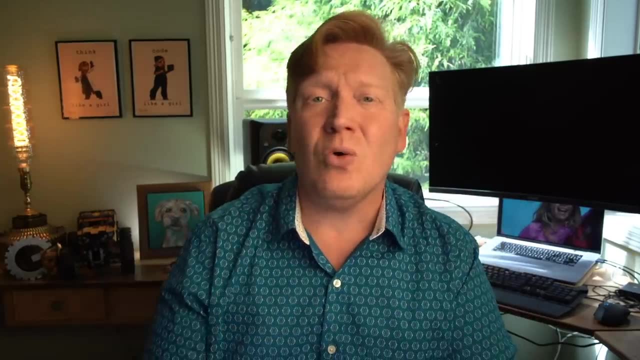 front of a building and it hides all of the mechanics of the building inside: the insulation, the rooms, the plumbing, the electricity and the basement and all that stuff that you don't want to see is hidden behind this nice facade. It's got a door and some windows and all of that looks 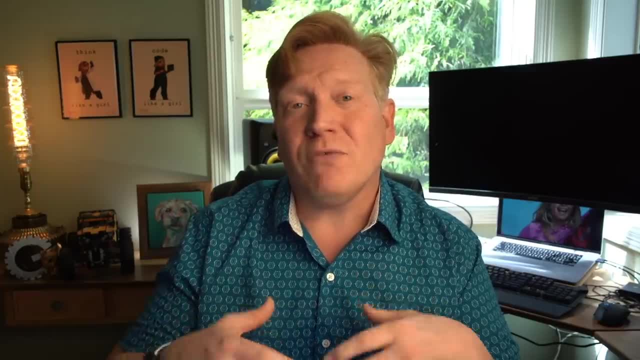 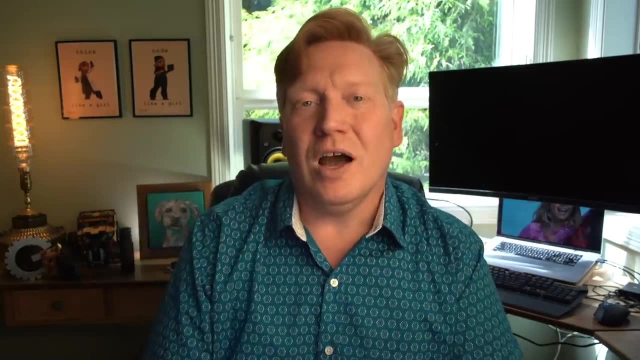 really pretty, got great curb appeal, And so, as a front-facing design, you've got to make sure that you're using it the right way, And so, framework creator, this gives you the facade pattern, gives you the ability to put a nice external veneer on your app. Now, the example that they use in the book is a compiler, So a 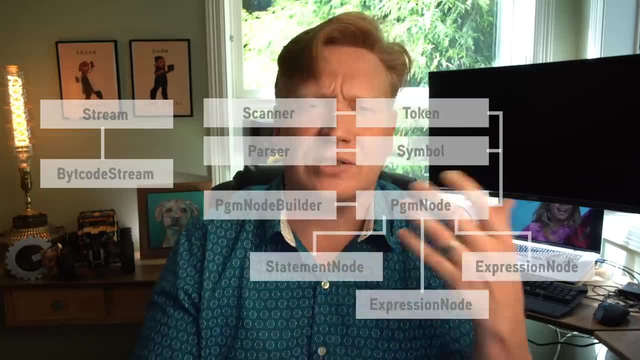 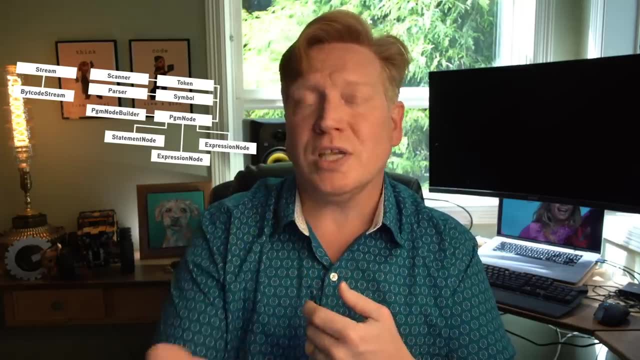 compiler has got all kinds of cool stuff inside: It's got a parser, It's got a lexical analyzer, It's got a tokenizer, It's got all kinds of fun stuff in there. But from a consumer standpoint, when you, as a framework creator, are thinking about your customer and having empathy for what? 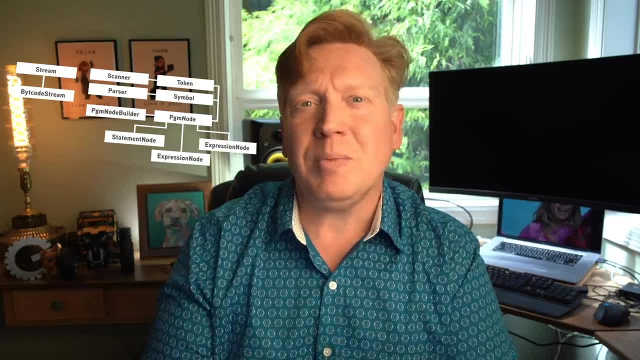 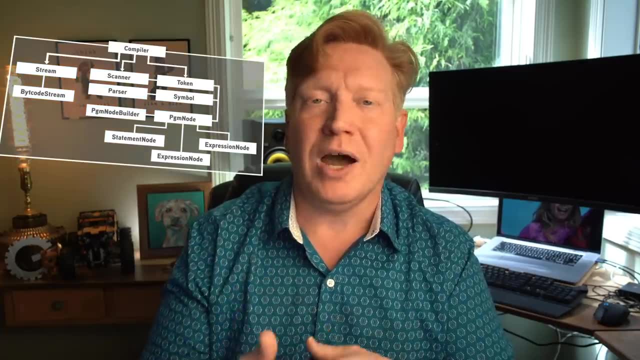 they want to do in their priorities. you're saying to yourself: oh, maybe I don't want to give them access to all the internals there, Maybe I just want to give them a nice compiler facade where they give me something, I compile it and I return it and away. 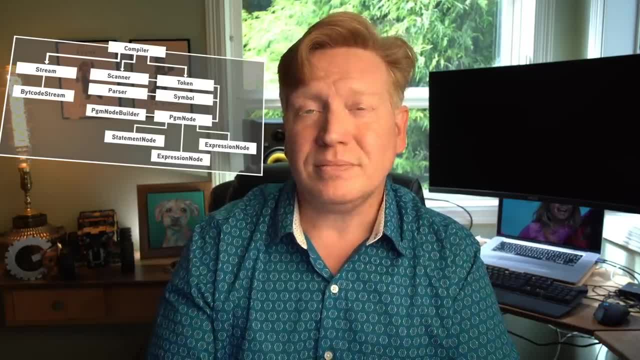 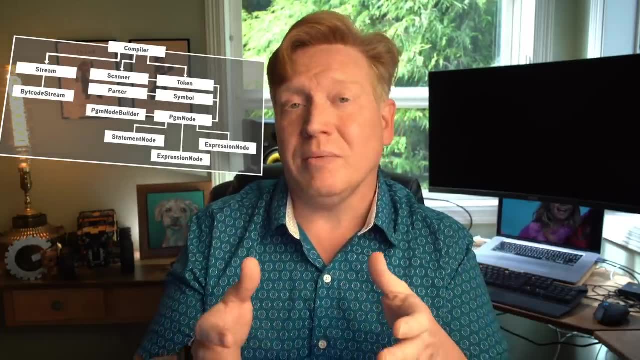 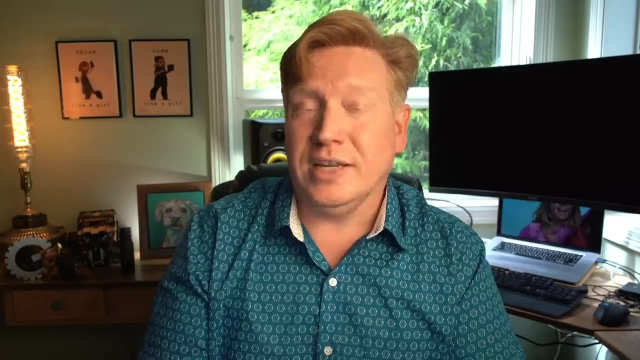 you go And I hide all those internals. So that's the big pro. It gives you and your consumer a nice interface And if you allow them, then if they want to, they can go around that interface and go and get to the interior if you so choose. Now the downside is you can have a leaky paradigm. 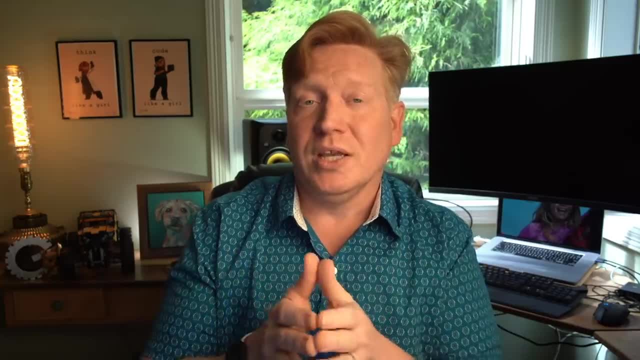 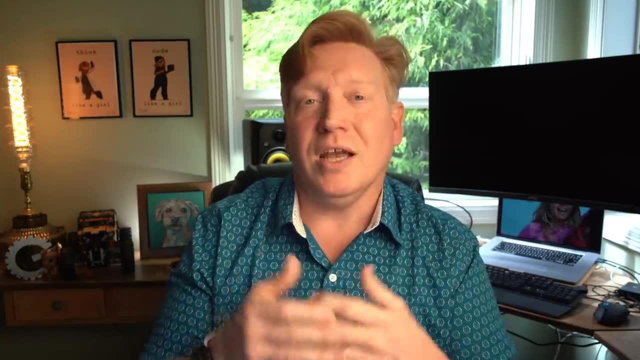 there You can have a leaky abstraction, In other words, that you've oversimplified. that compiler interface is so simple that it's not really usable and not really valuable, And that can be a problem. Another problem is over verticalization, meaning that you've created a facade that's so specific. 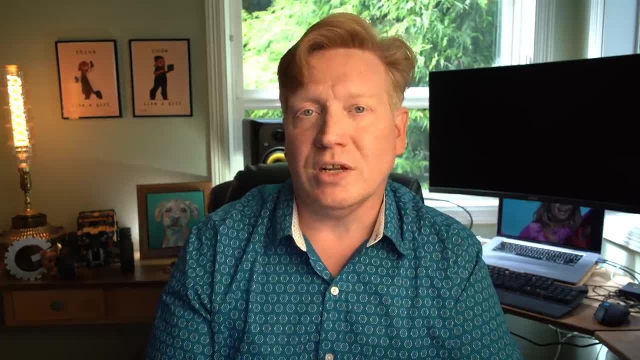 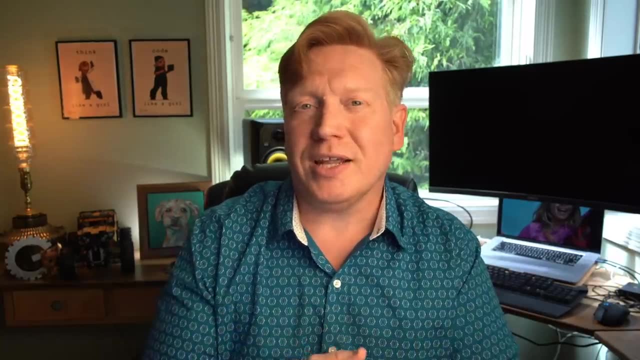 to a single use case that it's no longer generalized enough to be generally useful. So those are things to watch out for when you're using a facade pattern. So the next design pattern we're going to look at is the bridge pattern. I call it the. 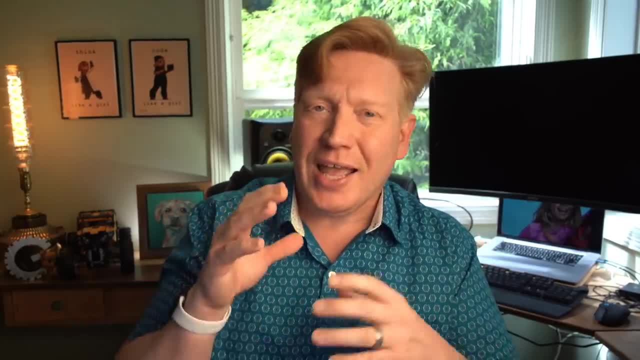 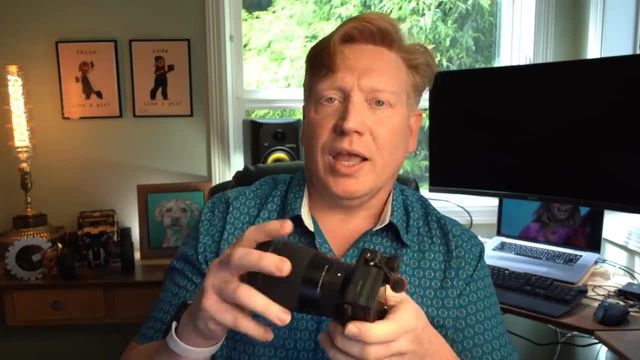 adapter pattern. but they've got a different definition in the book for the adapter pattern. But let me use a visual example on this one. So here is a Sony mirrorless camera, just like the one I'm shooting on right now, And it actually is two pieces right. So you've got the camera body. 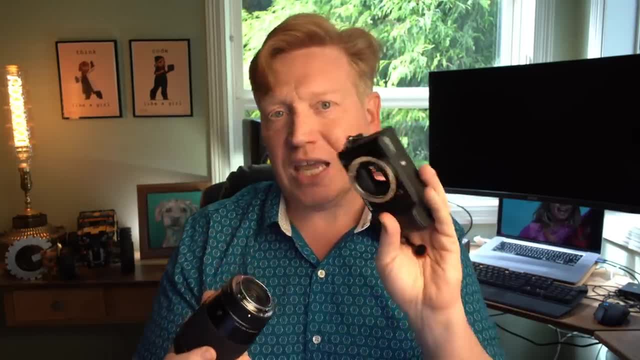 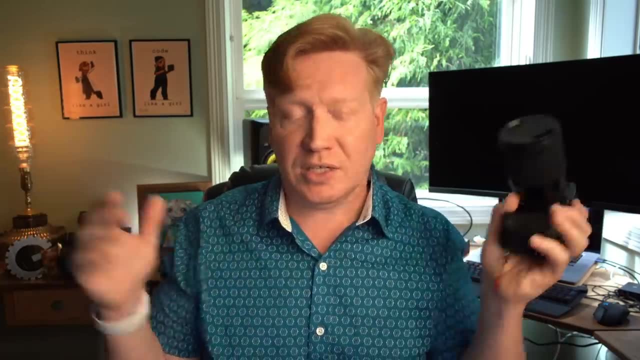 and then you've got the interchangeable lens And that allows this camera body to be multipurpose, right? In this case, this is a wide angle lens, good for giving nice big context like this. This is a 55 millimeter lens, which is a lot better for doing kind of headshots. 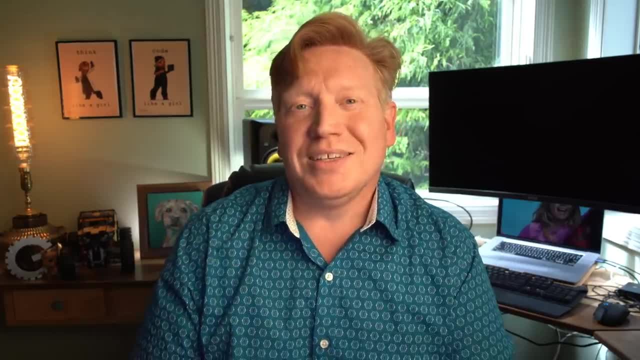 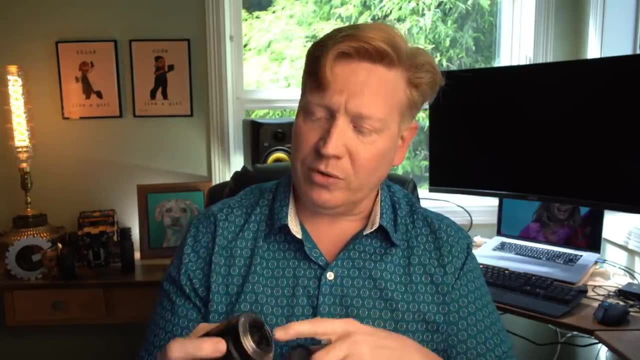 and portraiture And I use that when I'm doing zoom calls. So why that's important in this context is from the software perspective. you're doing a similar sort of thing. you're creating an API or, in this case, the API is this like connector here in software world. that would be. 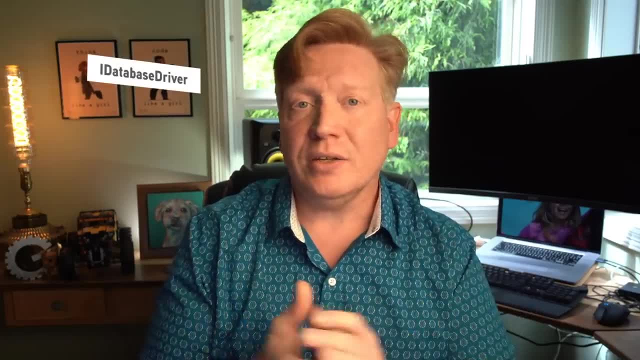 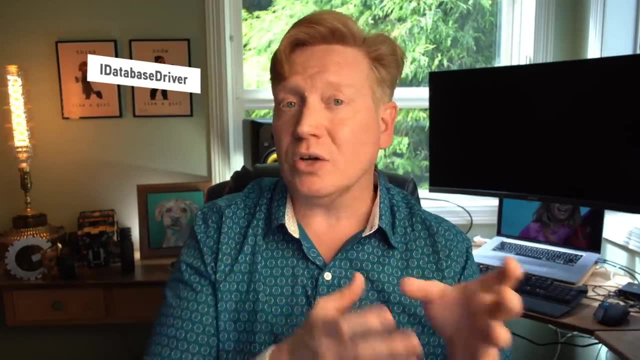 an interface, right. And so now on the server side you might have that database driver that we talked about before. you'd have an abstract interface for your database driver And then you'd have concrete implementations for, say, Mongo or Dynamo. 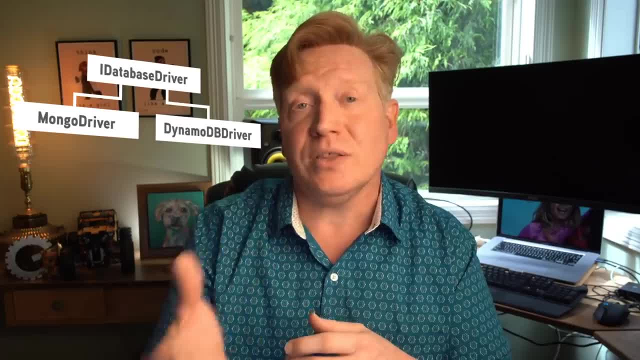 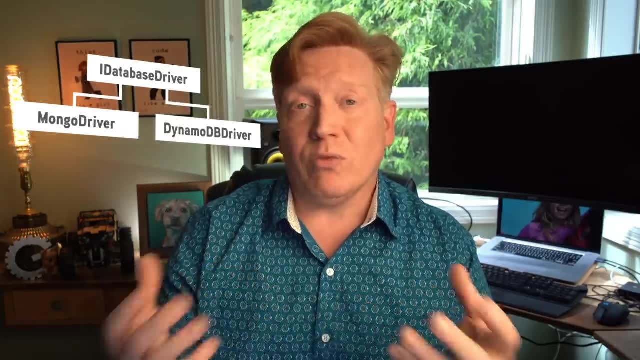 DB or whatever else you're going to get into. And that's a great thing about this pattern is it allows you to create a product that's usable by a wide variety of customers in a wide variety of situations. Similar sort of thing on the client side you could do an analytics abstract interface. 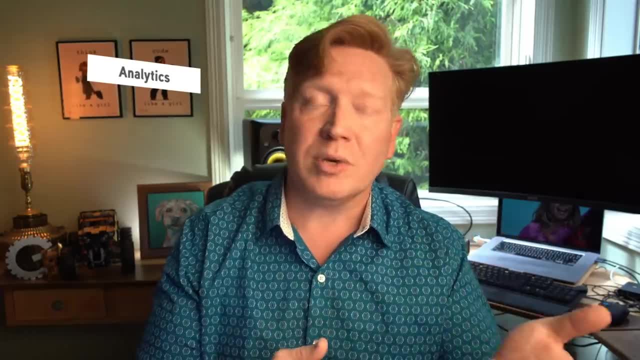 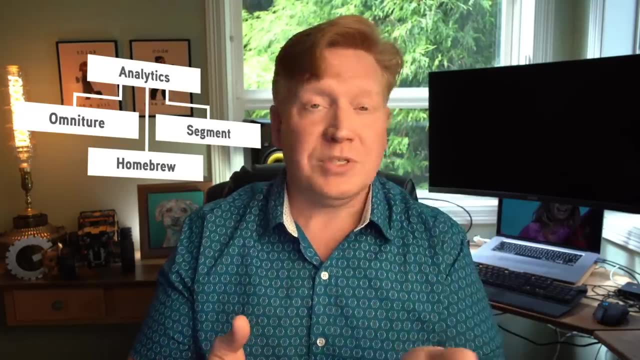 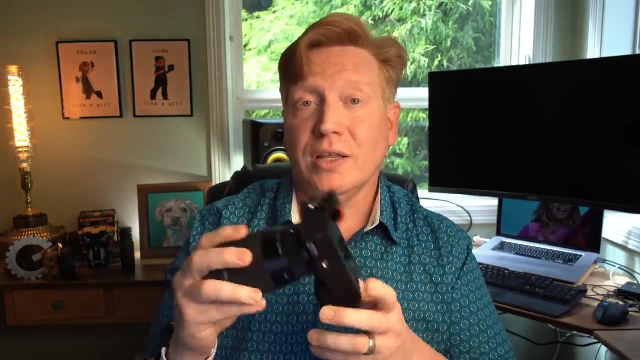 and then have concrete implementations to go to something like Adobe's Omniture or segment or your own in house homebrew, whatever you want, And that can work both on the website or on mobile. The problem is, the big con on this one is when you use it too much, right? So in this case there's only one. 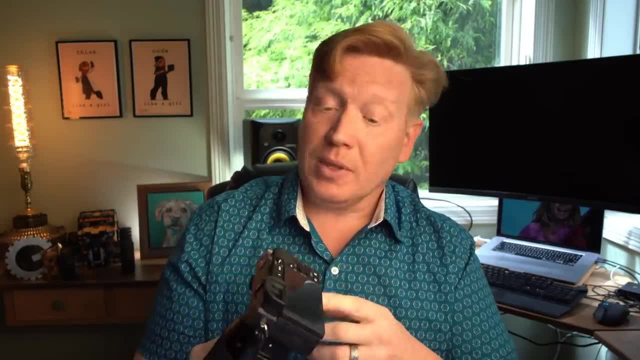 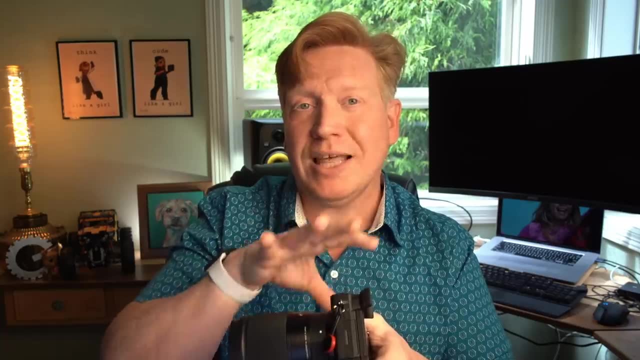 extension point to this camera and it's this interchangeable lens. So when you didn't go and go create modules for this little dial here or the eyepiece right, they use the that pattern judiciously, So you should do the same when it comes to your software. Don't overuse this pattern. 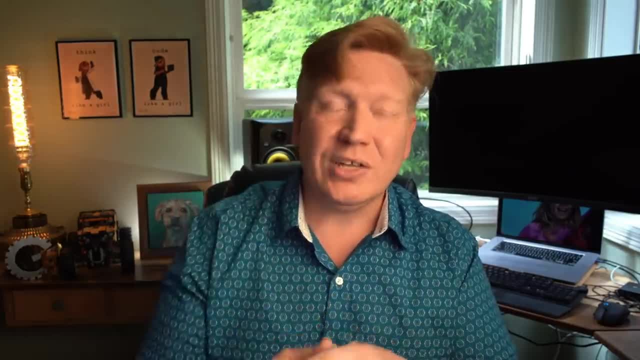 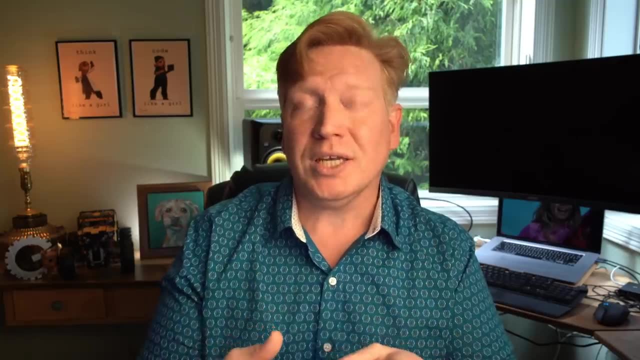 And the great thing about it is, you can also bring it in later, And that's what you can do with a lot of these design patterns. you don't have to start out of the box by creating the world's most modular system, get something working And then, when you 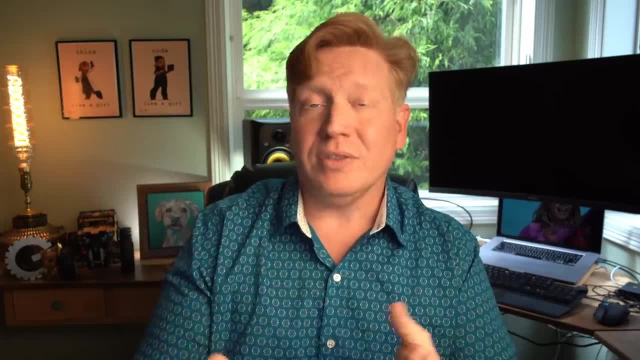 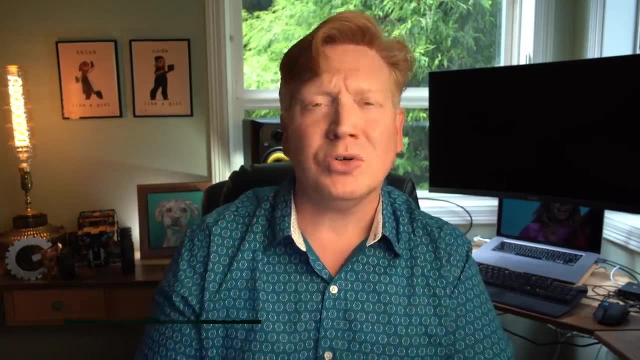 see the points where you need modularity and this bridge pattern, then go bring those in. The fourth pattern we're going to look at is the strategy pattern, And it's one of my personal favorites. So let's take a scenario: you've got this piece of furball code that's going to go and 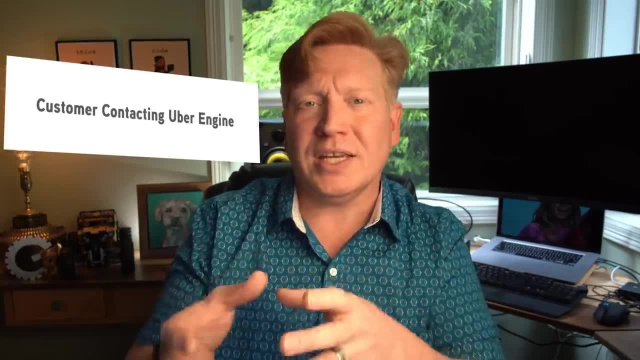 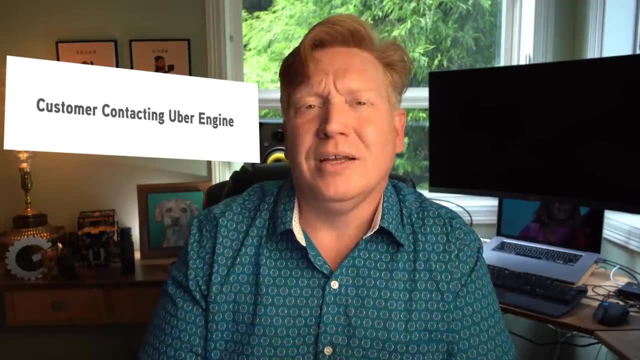 find a bunch of customers, filter through them and then send out email and text notifications to them, And nobody likes working on this piece of code, since doing multiple things and it's just a hairball. You can use the strategy pattern to significantly clean this up, And how you do that is you go and 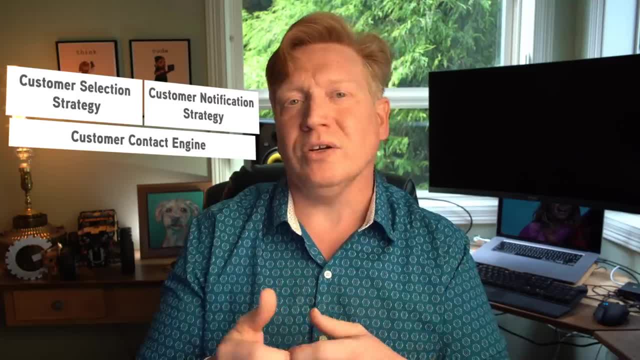 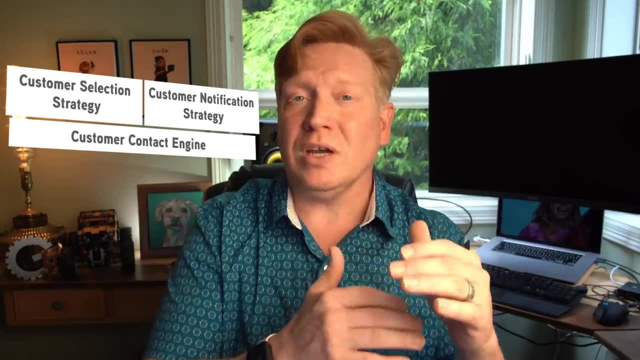 take the mechanics of getting access to the customer records, sending out the text and emails and then creating that as an infrastructure layer and then factoring out the filtering of those customers into one strategy, which is the strategy that helps you go find the target customers. you 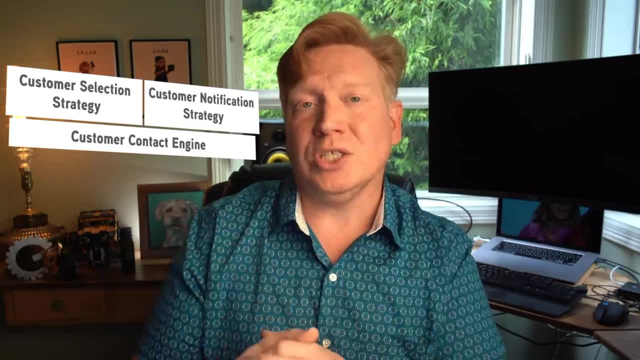 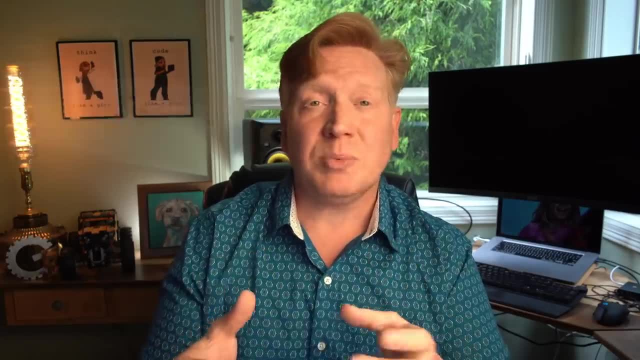 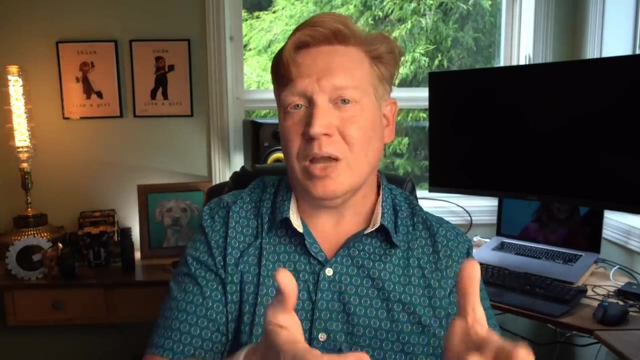 want, And then the notification strategy as a different strategy, And that helps you decide when and where and how to do that. So that's one of the things that you can do, And then you can actually use that library or that system in a whole bunch of different scenarios and it becomes 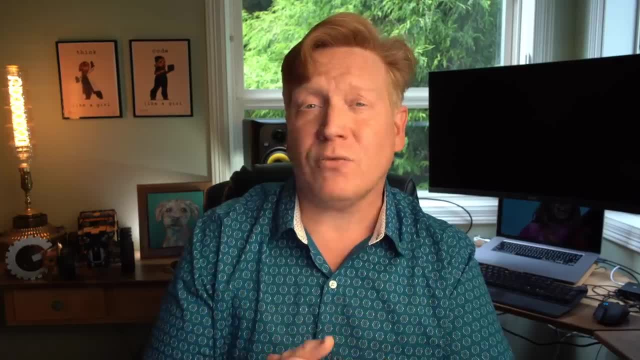 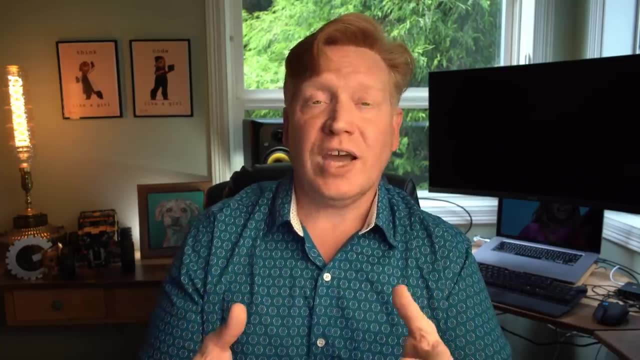 much less of a hairball. So one thing you got to look out for on this is always make sure that you have decent default strategies. So in the case of our refactoring, we go and take the existing logic around the customer filtering and then we go and take the existing logic around the customer. 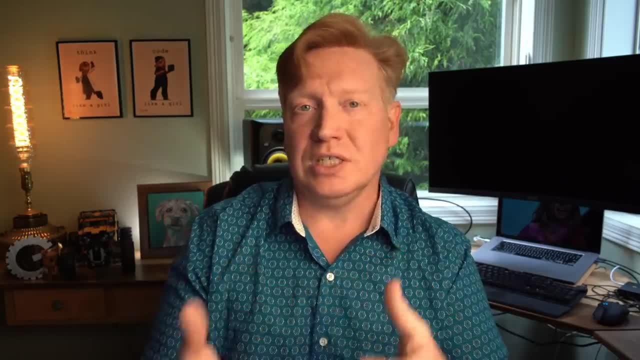 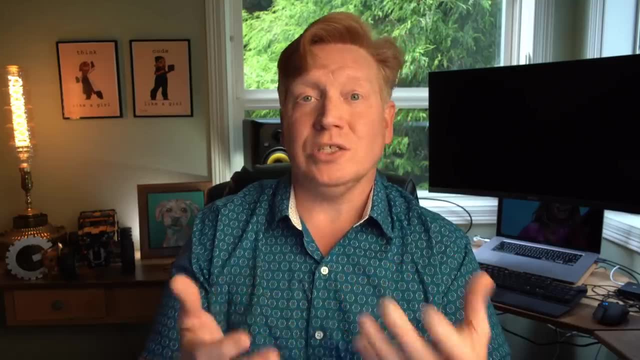 filtering, and then we go and take the existing logic around the customer filtering and then we- the customer- send outs and turn those into the default strategies And then later on people can extend them. Otherwise you get a system where by default you're asked to do a lot up front. 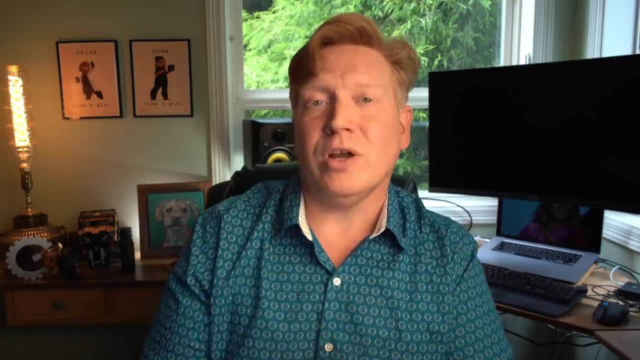 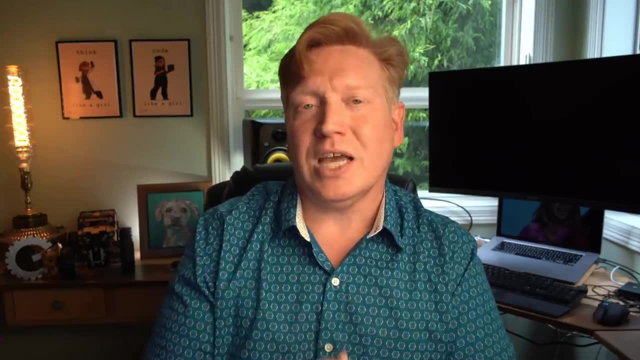 and no customer wants to do that. I want to go and take your library off the shelf, just use it right away And then, if it doesn't match what I want to do, look and see what the extension points are that I can tap into to modify the behavior to where I want it And the strategy pattern makes. 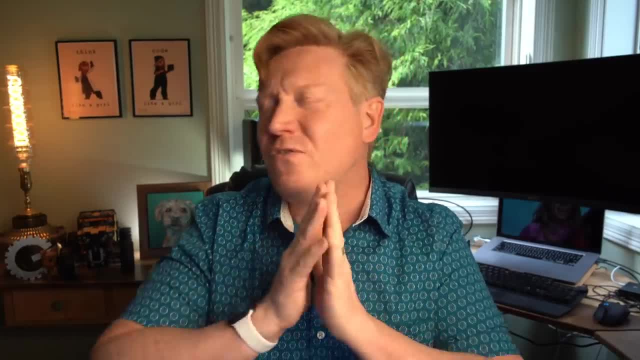 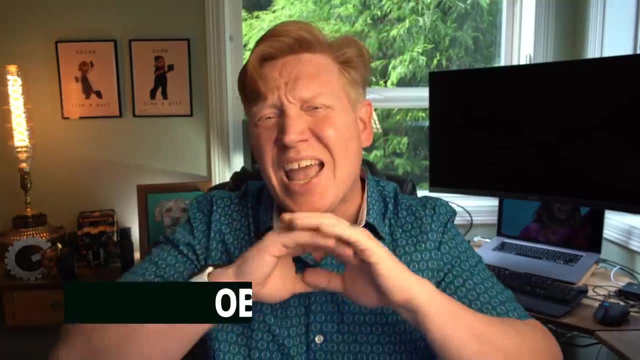 a great way to do that. The fifth pattern we're going to look at is my favorite of all of the patterns And it's the observer pattern, or what we've come to know now as Pub Sub, because it's everywhere. It's on the server as message queues between applications. it's on the client as 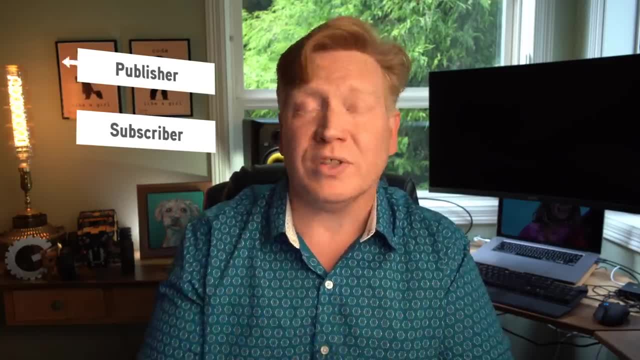 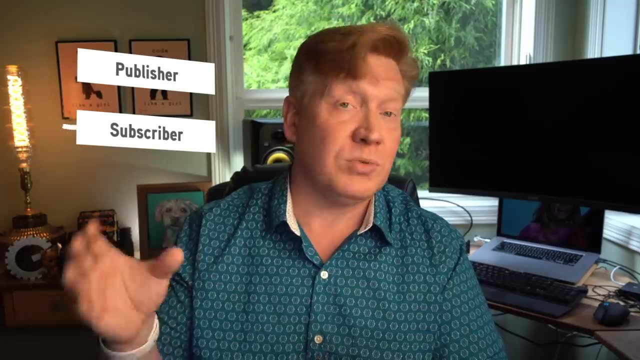 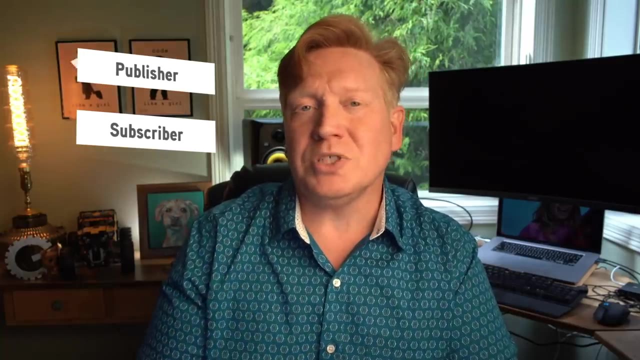 eventing systems. Pub Sub is everywhere And there's a good reason for that, because it allows for loose coupling between the publisher that's creating events and the subscriber or subscribers that are listening for those events, And you can use it anywhere. Now the con on this particular. 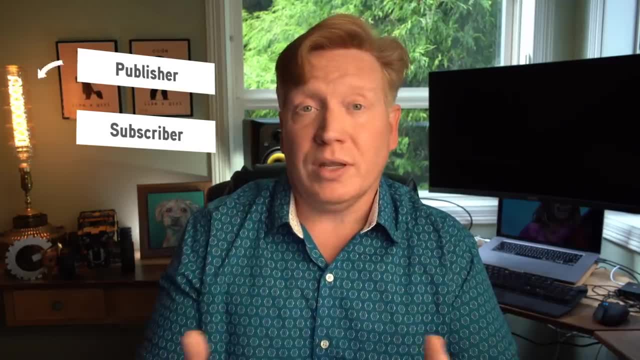 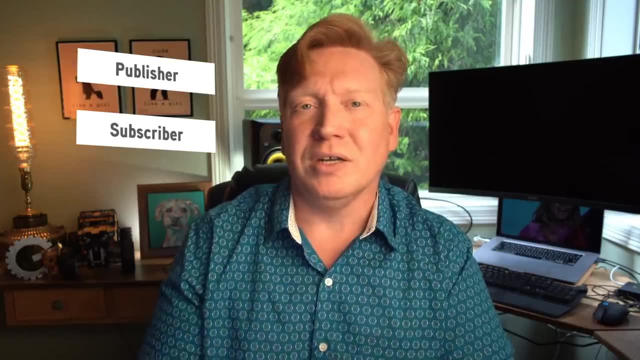 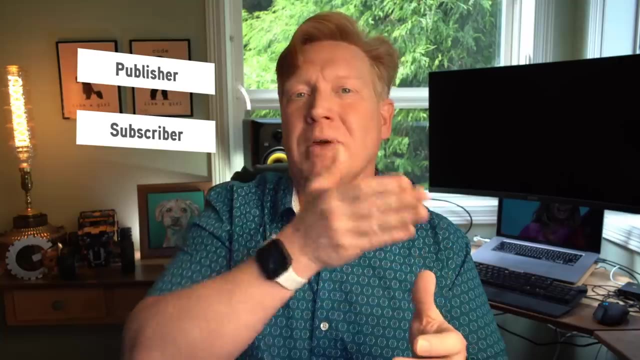 pattern is that you can go overboard with it. If everything is communicating by events, then you can get into nasty event loops and it gets very hard to debug. One thing publishes an event, it goes to another object which in turn publishes its own events, and it ends up kind of coming back. 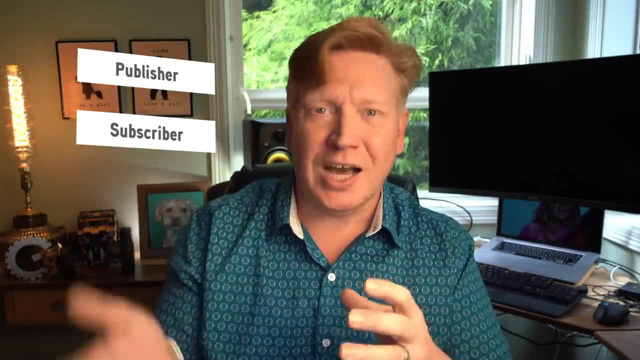 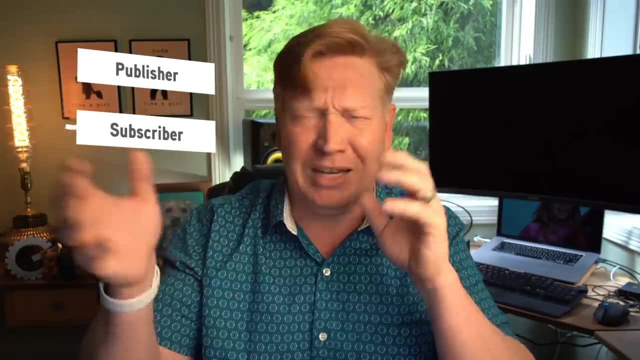 around to the original event, which ends up creating more events, and on, and on, and on. And then you know you got a serious problem where you're ending up adding in booleans to check whether you're emitting events, and it just gets hairy. 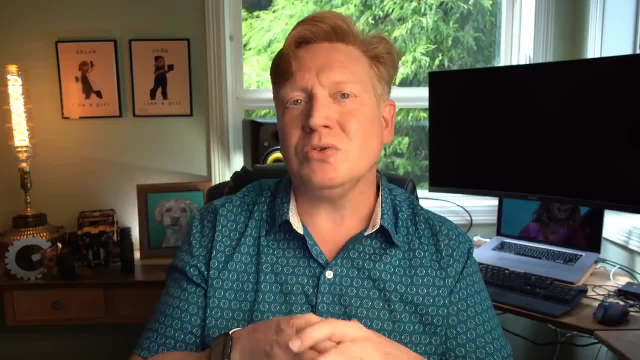 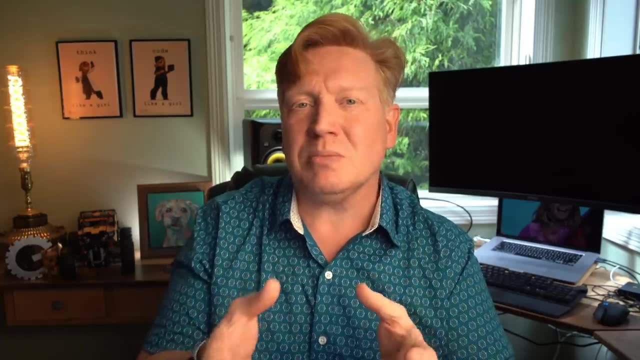 So there's a couple of solves for this. One is: don't use the same message bus for everything. have a specific person purpose for each message bus And then, to you know, keep these systems localized. you know if you're on the client, you've got a button and it's an emitting an event. 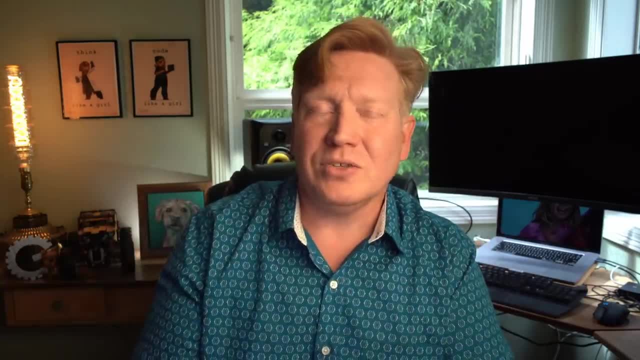 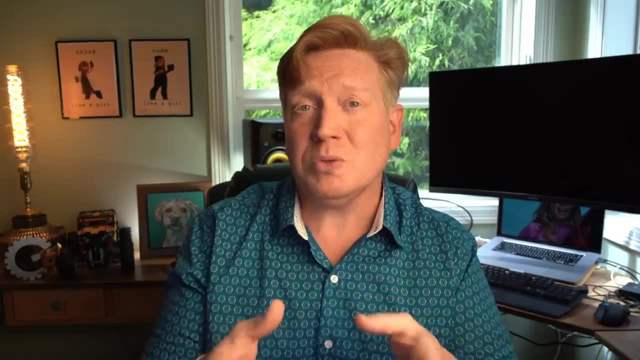 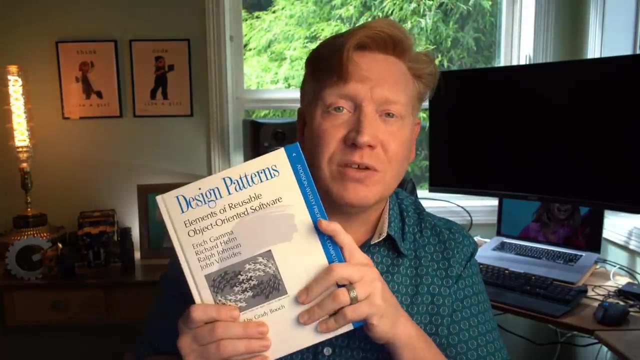 that's good. That's all you need. You don't need to go beyond that. So again, as with all of these patterns, use them judiciously, but use them because most people understand those systems when they see them. This quick tour of five types of design patterns: There are, I think- almost wow- 20 or so different.